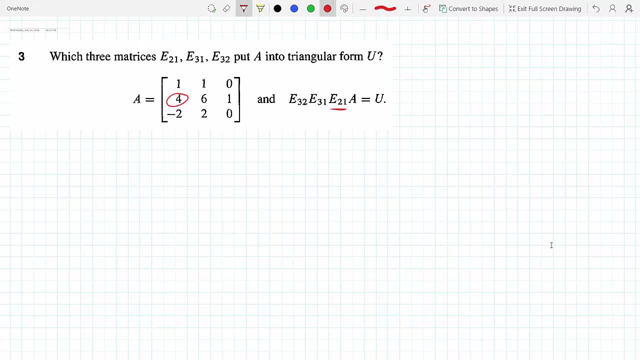 So it has to be an operation E21 between row number 2 and row number 1.. So, no, yeah, you just follow this. you know this is So. what I have to do is I would have to do a 4, negative 4 times row 1 plus row 2.. 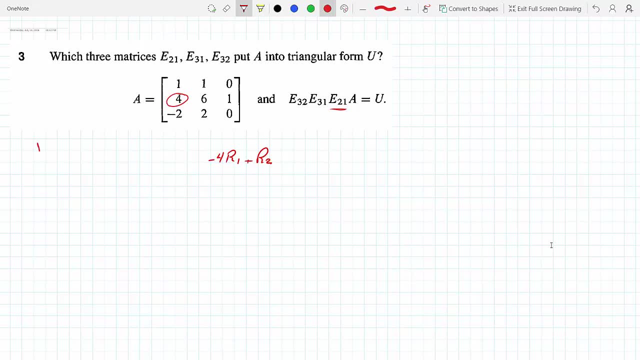 And what would that get me? That would get me. so we have 1, 1, 0.. So I start with A 1, 1, 0.. And what would that get me? That would get me. so we have 1, 1, 0.. So what I have to do is I would have to do a 4, negative, 4 times row 1 plus row 2.. 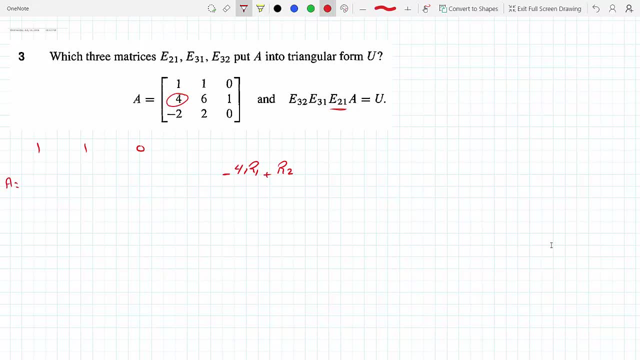 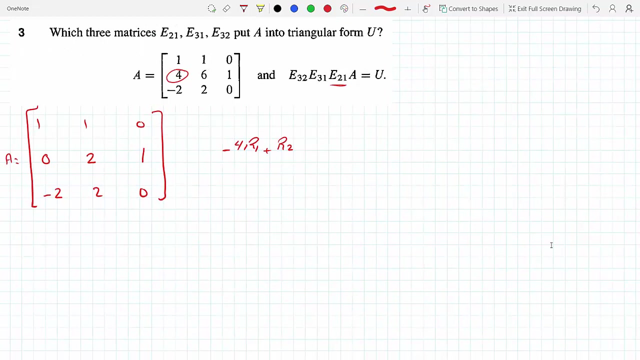 And what would you get here? You would get 0 on the first one. yeah, Minus 4 plus 6, you would get 2.. And here you would get 1 minus 2 to 0, right, 1, 1, 0. Okay, good, Now this is here E21.. So what we do is we apply this E21 on the identity matrix. 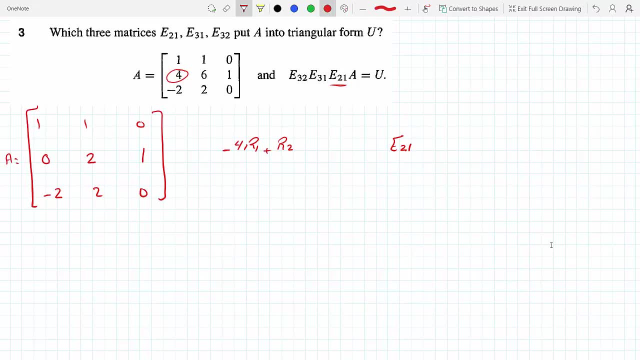 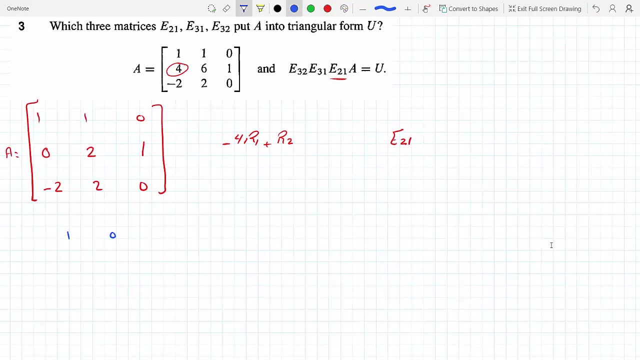 So the identity matrix is 1, 0, 0, 0, 1, 0, 0, 0, 1.. And if we apply E21 here, that we applied up there. so this is the identity matrix. what do we get? 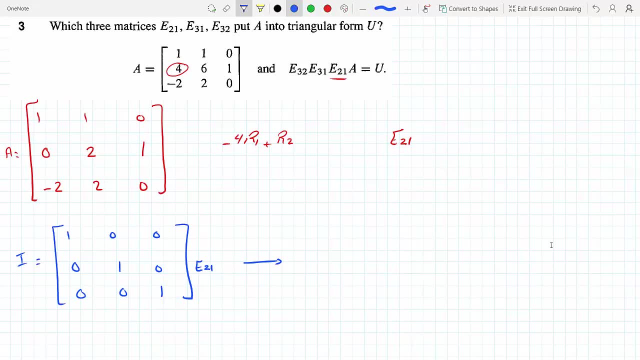 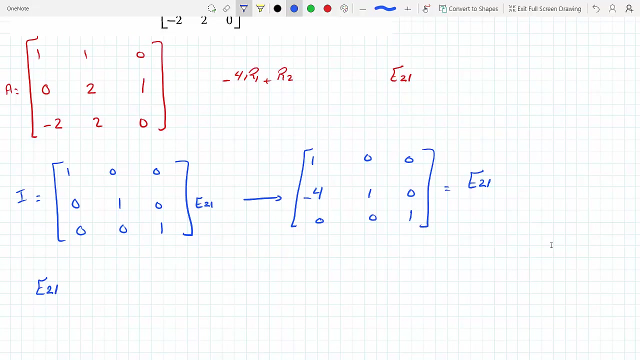 Minus 4, R1.. So we would get minus 4 here, 1, 0.. And these two stay the same. This is this is E21.. Okay, and now I take E21 times matrix A And I multiply them. 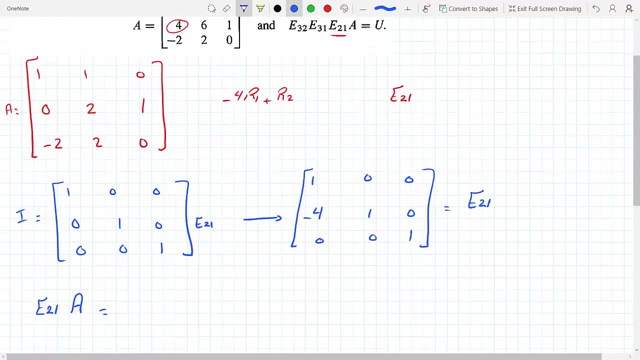 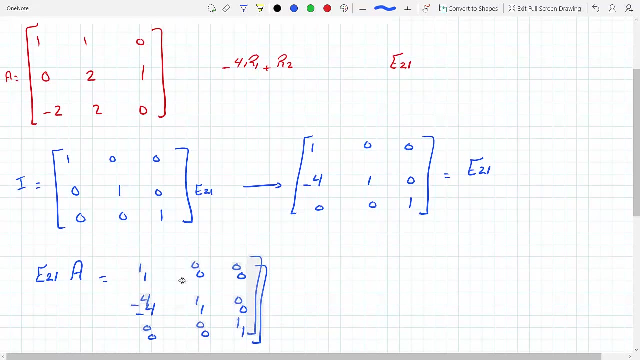 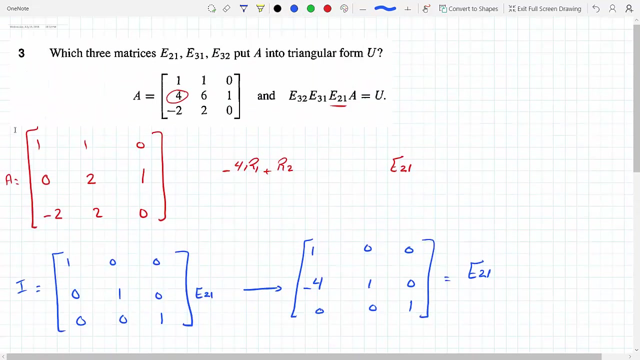 So let me, let me copy and paste here so I can make this, Okay, Okay, quicker. so if I do this copy here, so this is E21, and I'm going to multiply it by matrix A, which is this red one here? no, not this. this already changed. this is no longer A. 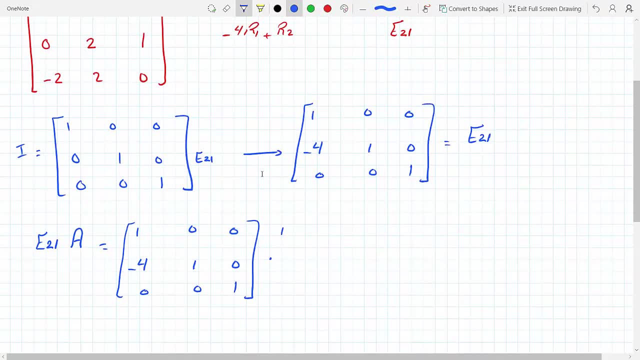 A is 1, 1, 0,, 4, 6, 1, and minus 2, 2, 0,. hold on, let me open the door, Okay. so okay, let's use the calculator on this. yeah, because you know how to do matrix. 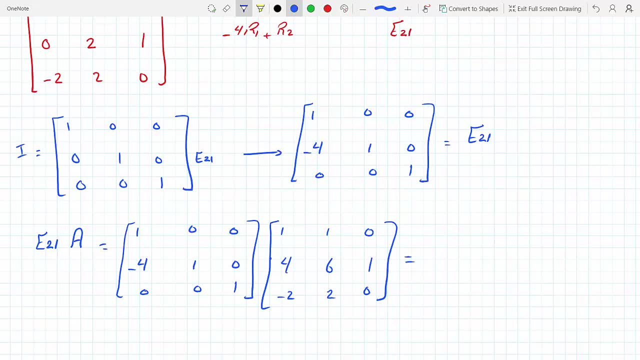 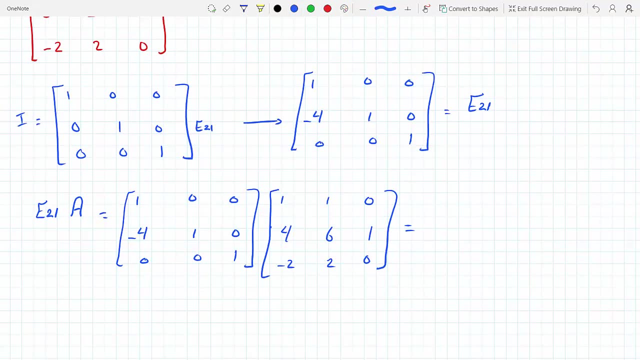 multiplication. Okay, so if I put this on the calculator, I will get one second: 1, 1, 0, 0, 2, 1, minus 2, 2, 0, this is E21.. 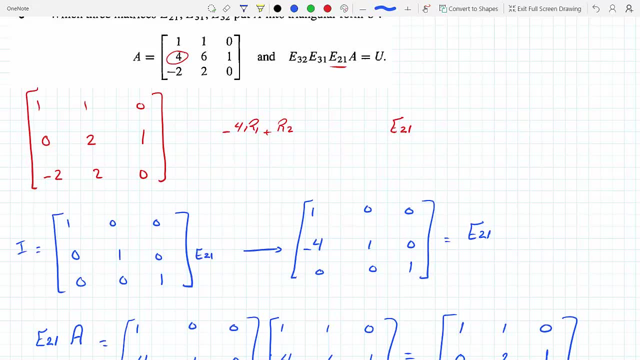 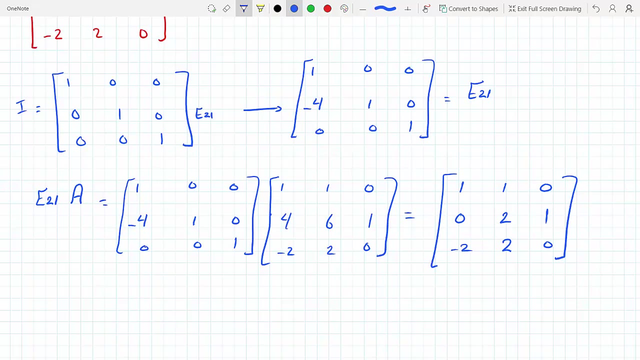 I'm looking for E21, A times E31, so now I move on. could you, could you hear me? Yeah, I hear you, Yeah. so I multiplied E21 times A and I got this answer. okay, Okay. 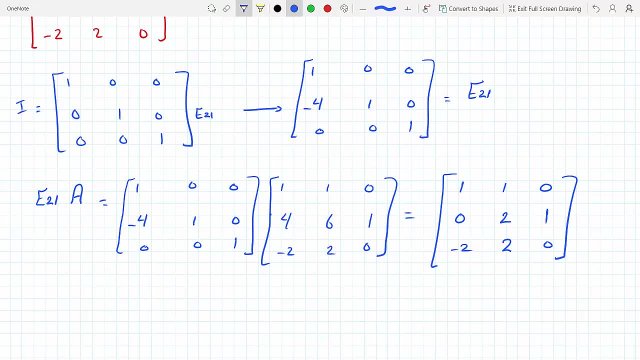 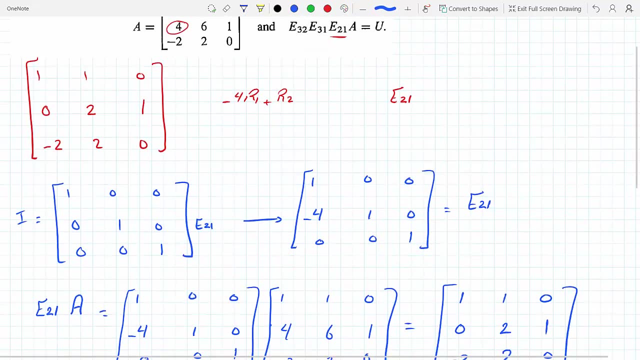 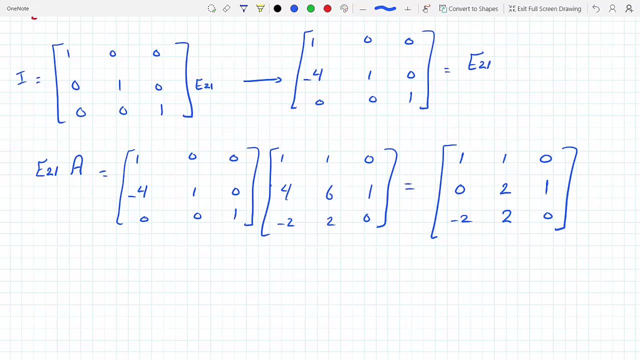 Oh wait, wait, you multiplied, or you? oh yeah, yeah, yeah, yeah, Yeah, I multiplied. Okay, now E31, so now we go back and we do the same thing for E31, mm-hmm, so we're gonna. 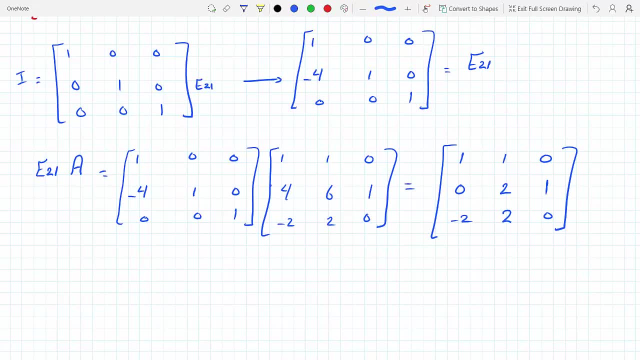 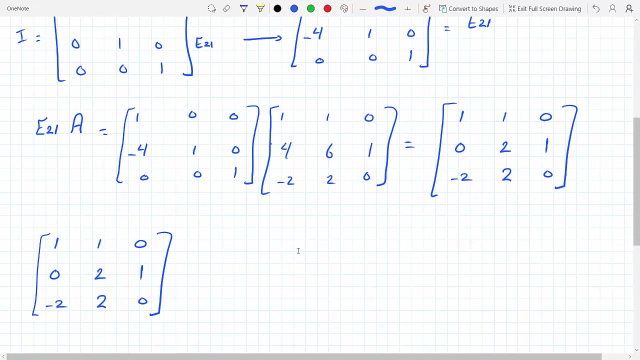 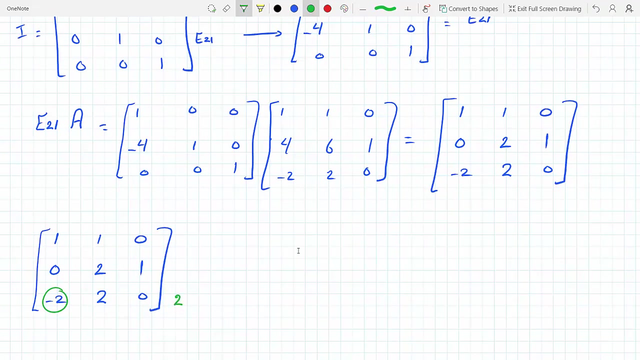 apply row operation 31 on the result. so I'm gonna take this matrix here copy. I'm gonna put it here. And now I need this guy to be a 0,, so 31,. so that's gonna be 2R1 plus R3, and if I do, 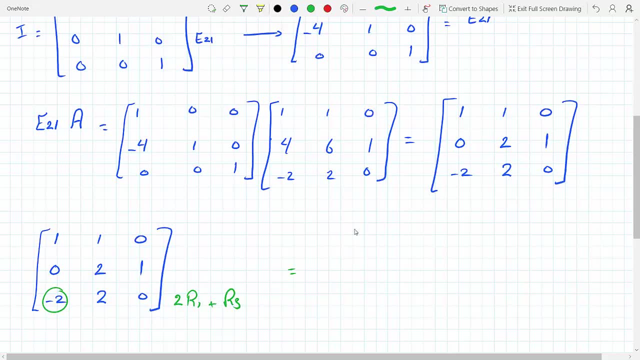 that, what do I get? Well, I'm gonna get the same matrix, except the third row changed, so I'll just copy and paste B quickly, Okay? So, uh, then this will be uh 2 times 1,. this will be 0,. uh, this will be 2 plus 2,. 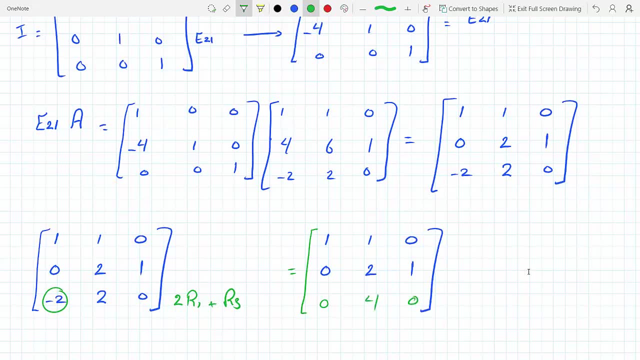 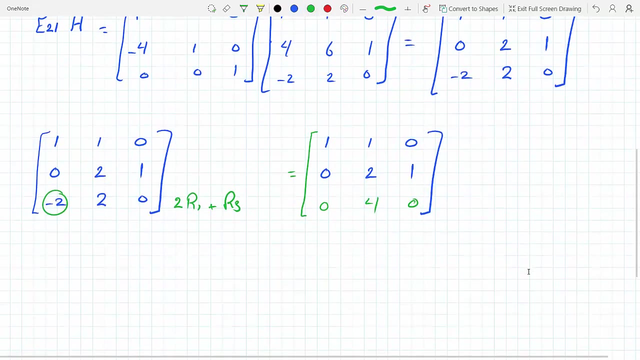 4, and then 0 plus 0 is 0. So I get this, okay, Okay. now, uh, how do I get so? now I apply E31 on the identity matrix. Okay, Okay, Okay, Okay. 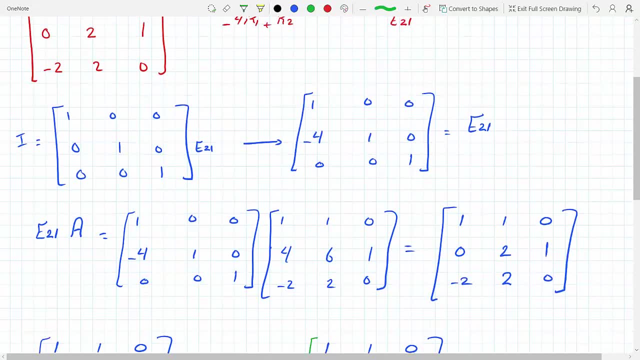 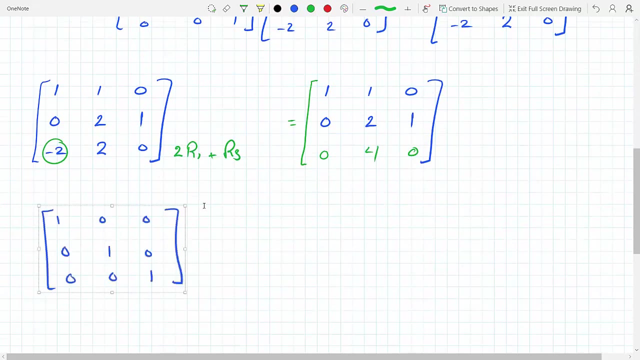 Uh, what's the identi- the? uh, let me, let me copy and paste the identity matrix here so I don't have to rewrite it. So, and with that same row, operation: uh, E31 will equal uh. so if I do, uh, I'm gonna. 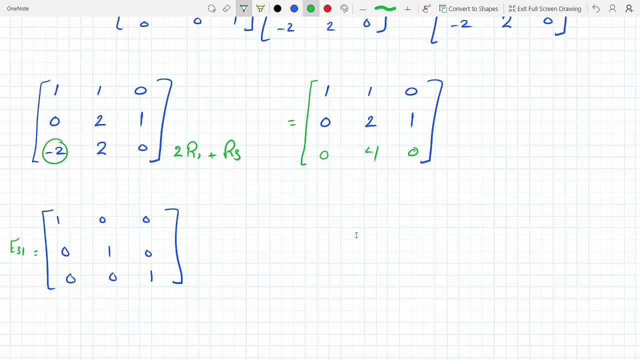 apply this on on B. Oh okay, So this will be E32.. So I'm gonna apply E31 on this matrix. on the identity matrix: Mm Uh, 2R1 plus R, so 2 times 1 is 2 plus 0, so this becomes 2.. 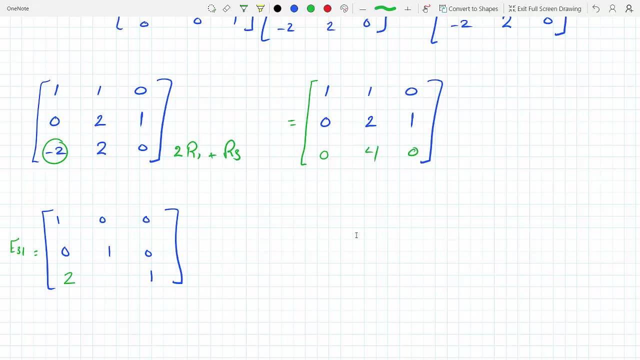 When I apply 2R1 plus R3 on this, this will stay 0 and this will stay 1.. So this is my E31.. So now I'm gonna find out E31. So I start to reverse from a backwards times e to 1 times a. so that's the next step now: e to 1 times a. 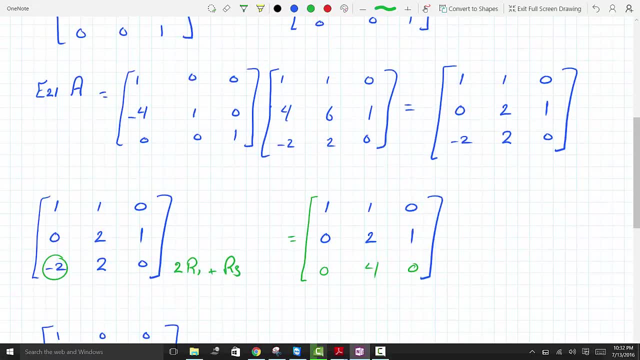 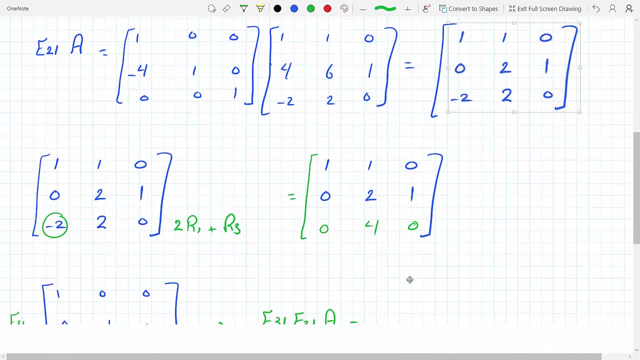 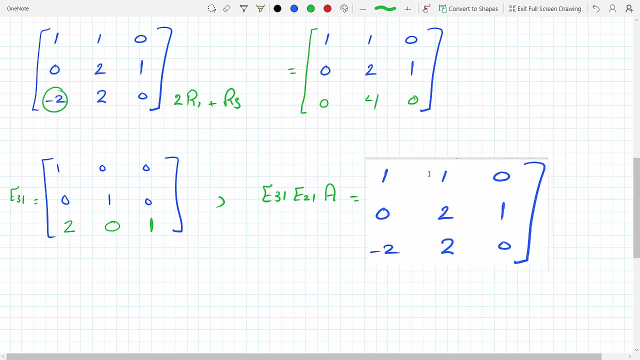 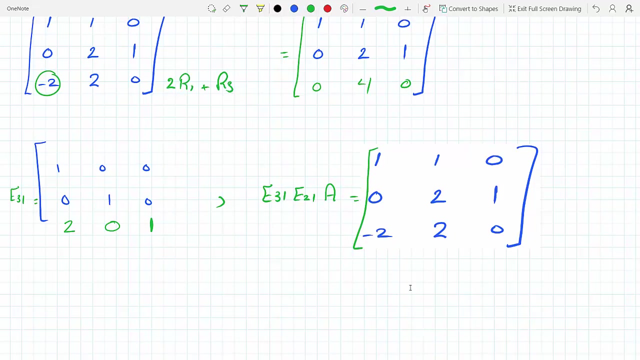 I already have that this is e to 1 times a here, so let me put this here: yeah, this is e to 1 times a, this is e to 1 times a, and I'm gonna multiply this by. why did this shift by e3 one? e3 one is 1 0 0. let me just write it: click 0 1 0, 2 0. 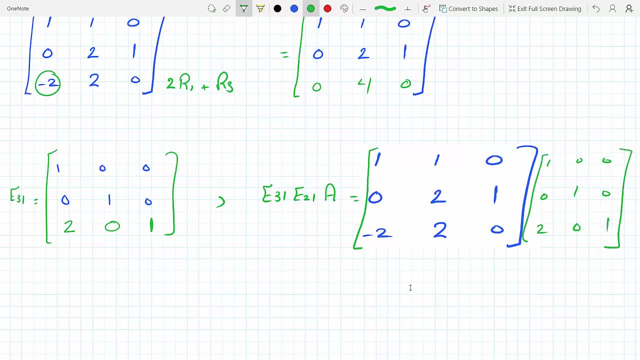 1 And you do this on the calculator And you get E21A. This will be one second. Okay, E31 has to come before I reversed them here. Sorry about that. This guy, This, you get my idea. This guy has to be here and this guy has to be here, Okay. 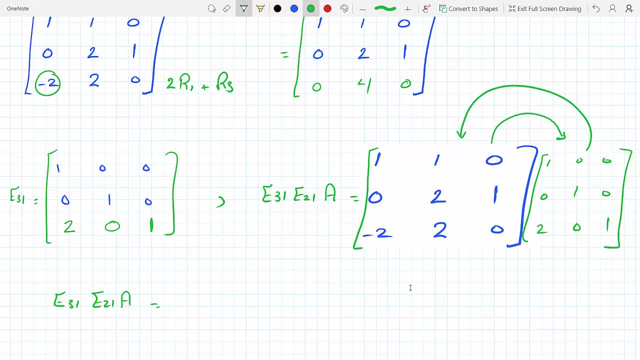 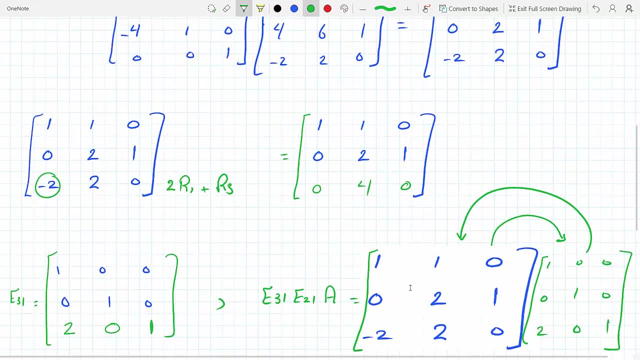 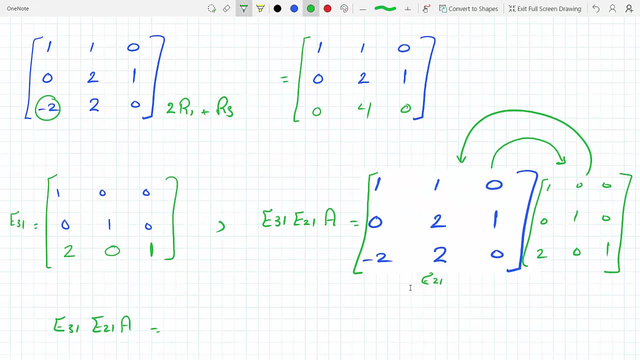 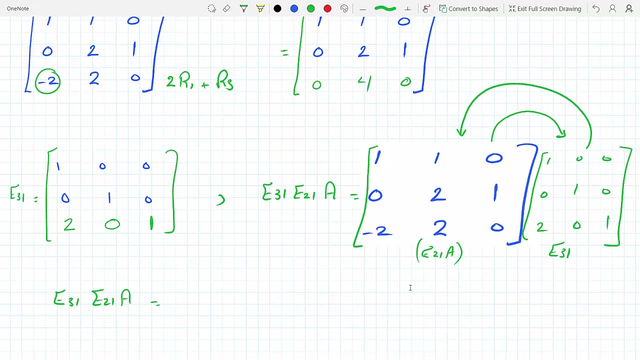 So just flip it, Because this here is E21 times A. Right, E21 times A is 110.. Yeah, This is E21A And this here is E31.. So they have to be flipped. So, anyways, when you flip them, you get 110. 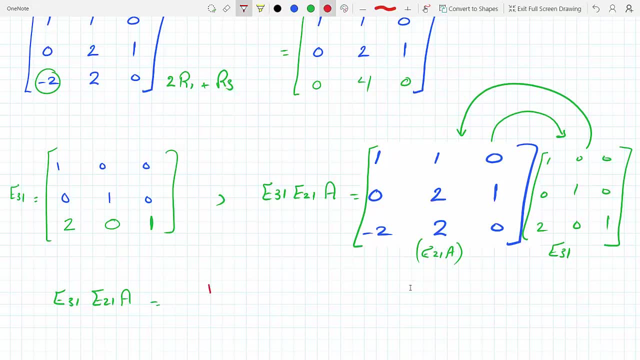 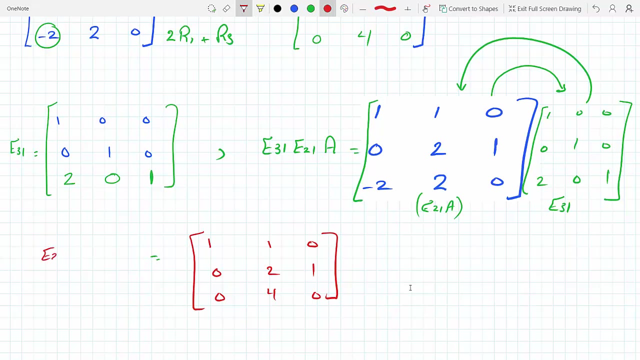 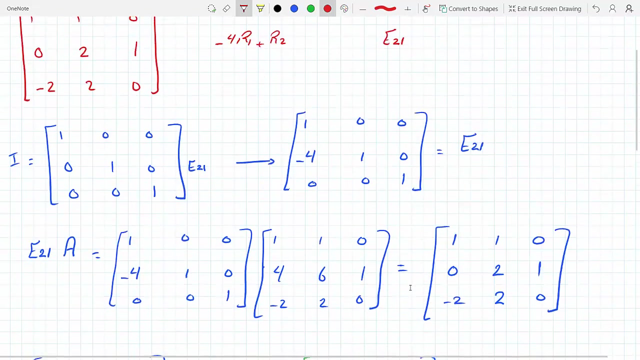 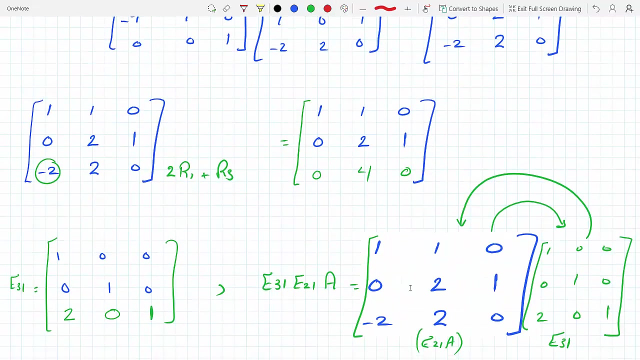 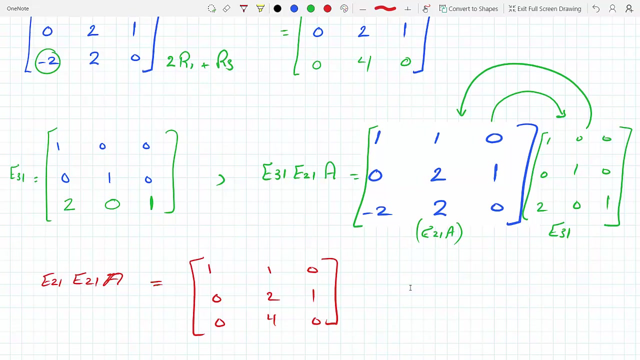 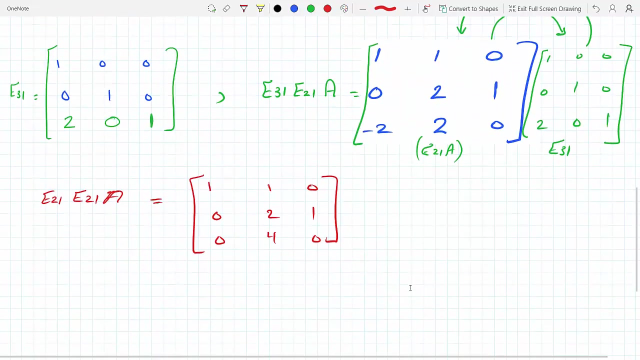 Let me change the color here: 110,, 021, and 040.. So this is E31, E21A. Okay, So we are up to this point. now We still need E32.. Okay, So E32.. What's E32?? I'm going to take negative 2.. Oops, Negative 2 times R2.. Plus R3.. 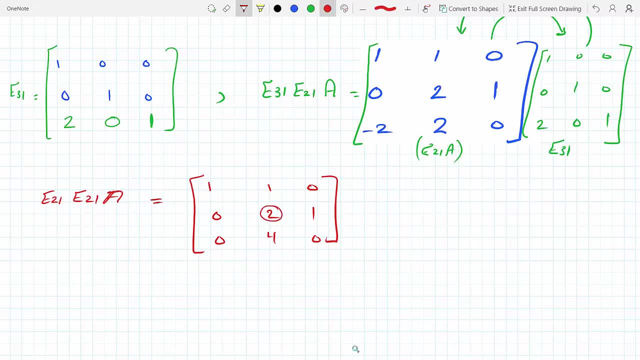 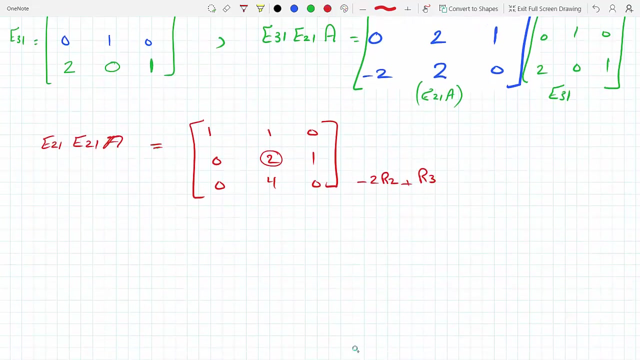 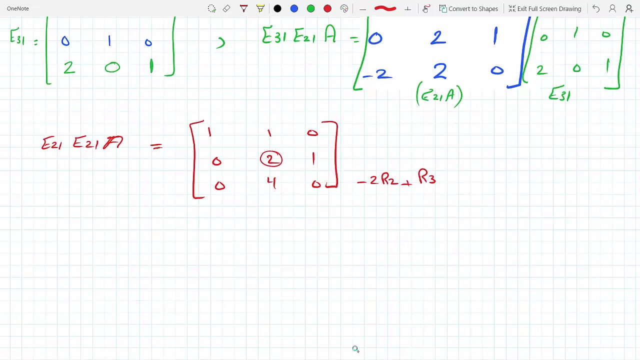 Why? Because I need to make this guy a 0.. So now we will do minus 2, R2.. This should go on row number 3.. Minus 2, R2.. Plus R3.. Okay, Okay. So now apply this on the identity matrix. So the identity matrix is 1, 0, 0, 0, 1, 0, 0, 0, 1.. 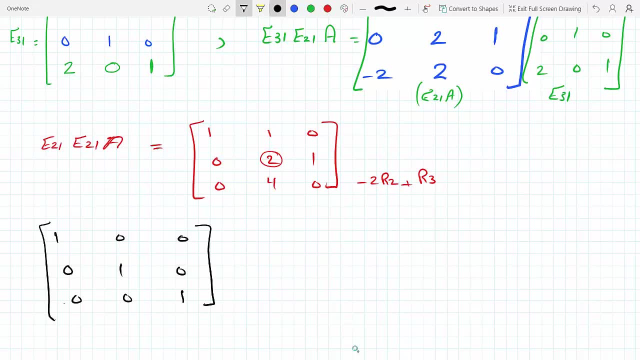 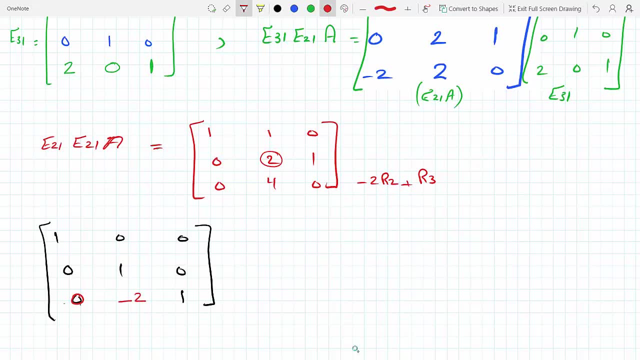 Okay, Okay, Okay, Okay, Okay, minus 2 and minus 2 times 0. 0 plus 1, this will remain 1. so this is my e 3: 2. what happens on the identity. make the result of what happens on the identity. 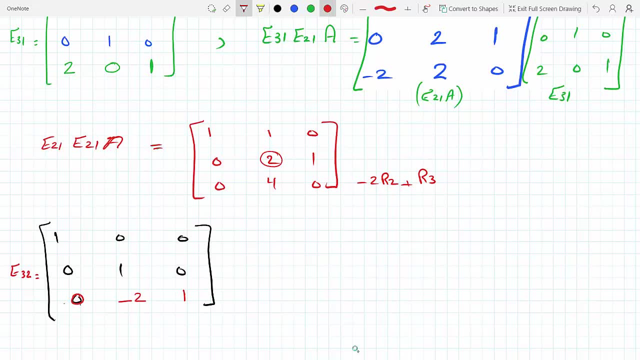 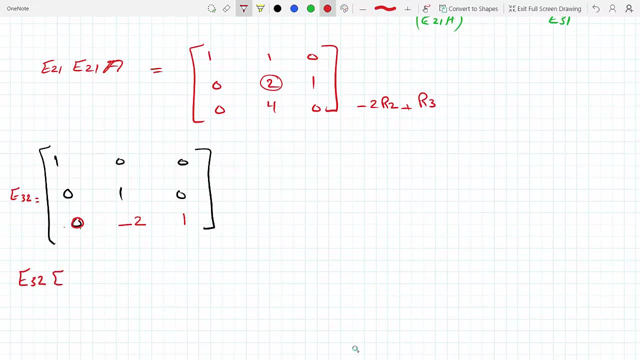 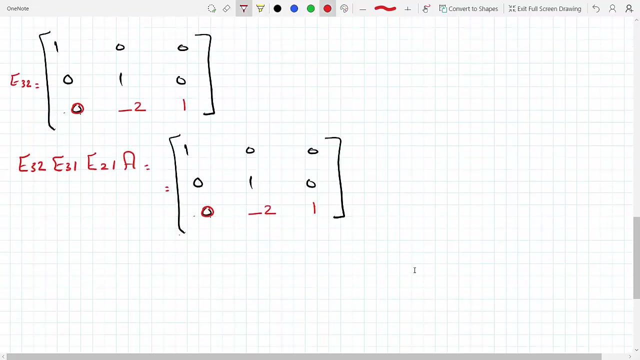 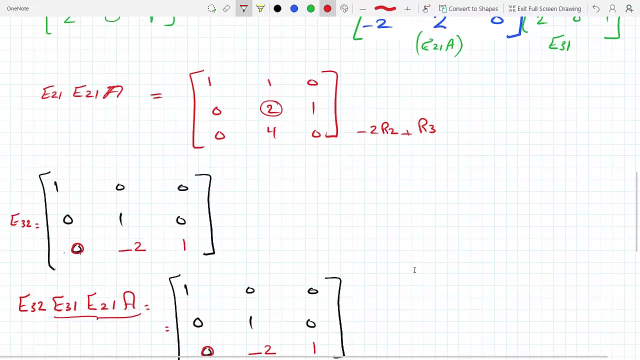 matrix is your elimination matrix. okay, and now, finally, I get my e 3: 2 times e 3, 1 times e 2, 1 times a. e 3, 2 is right here, this guy let's just put it here, copy paste, right, this is my e 3, 2, e 3, 2 and then my e 3: 1, e 2, 1 a I already have. 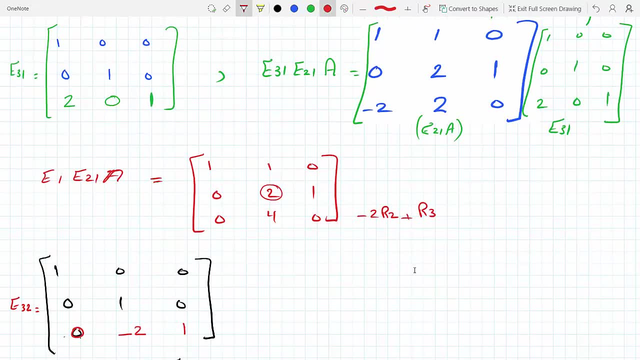 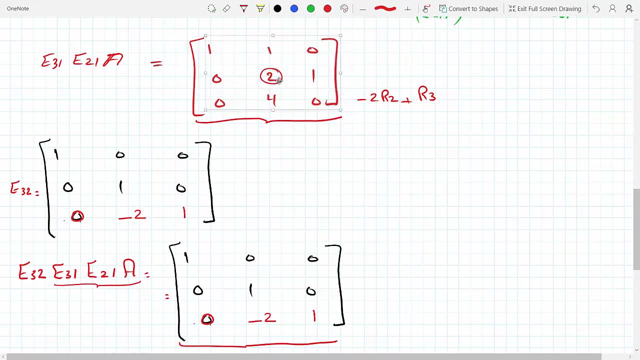 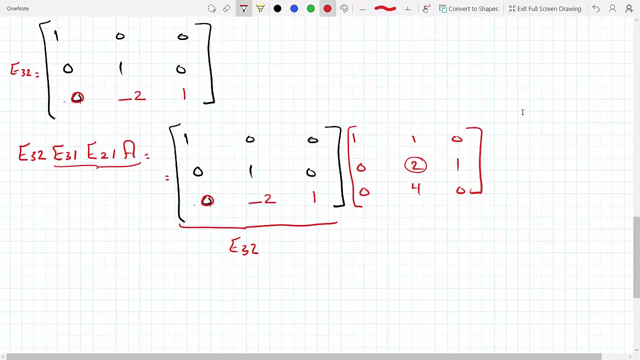 it. sorry, this is 3: 1. it's this right. so now this goes here and we multiply them and let's do that on the calculator and finally we get our u, which is e 3, 2, e 3, 1, e 2, 1 times a u is: